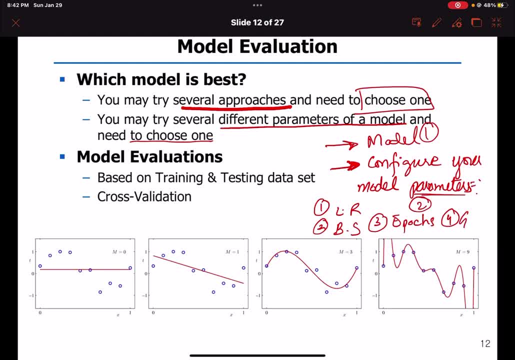 optimization algorithm. for example, you use gradient descent algorithm for optimizing or updating the weight values. so these are the parameter settings that we have to do. so the first approach is train and test data splits. you can evaluate your model based on that. and the second concept is cross validation. so we are going to study. 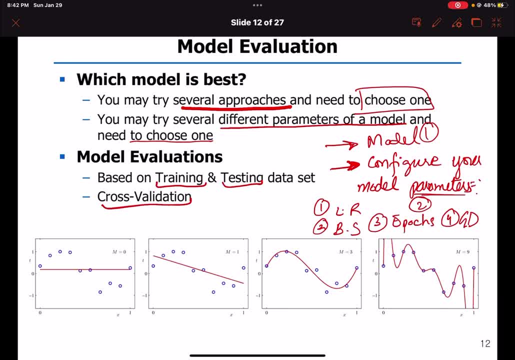 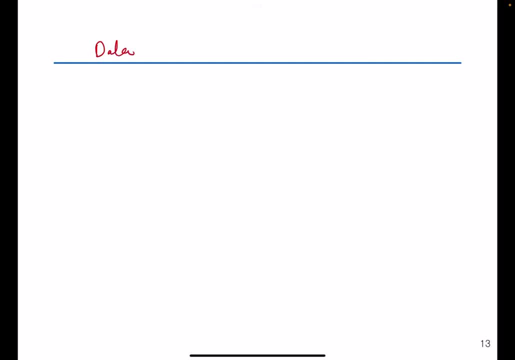 these two approaches. so first I will data set partitioning. I will explain data set partitioning. we already have studied this. I will take it a step further. so your whole data set is split into training data set, then your validation and then you're testing data. so these are the partitions. this 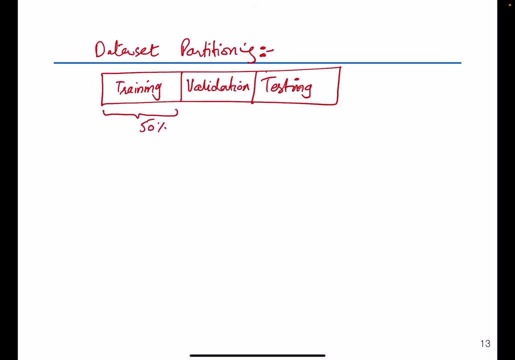 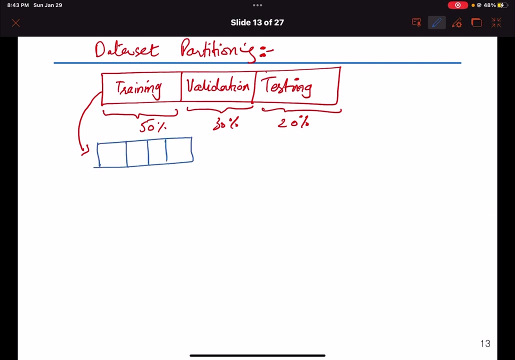 is 50%, nearly 30% validation and maybe 20% for your testing. so here your training. data is further split into batches. what are the batches? so, basically, one batch considers contains 64 data samples, then the next one 64 data samples, next one 64 and batch 64 data samples. so your whole data set. 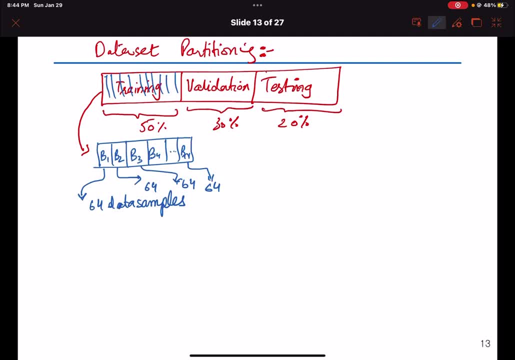 we know it is composed of data samples. this is we, how we organize the data in your batches. similarly will be the structure of your validation data. so if there are 64, you have to set best case 64 data samples for each batch in your validation data, as well as your testing. 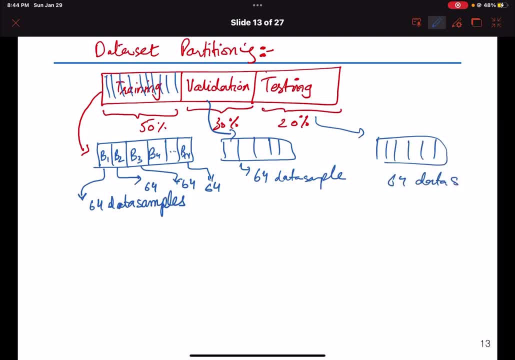 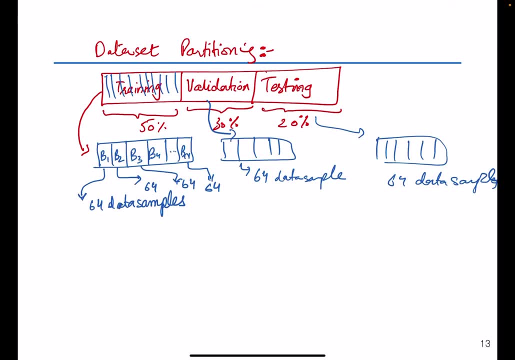 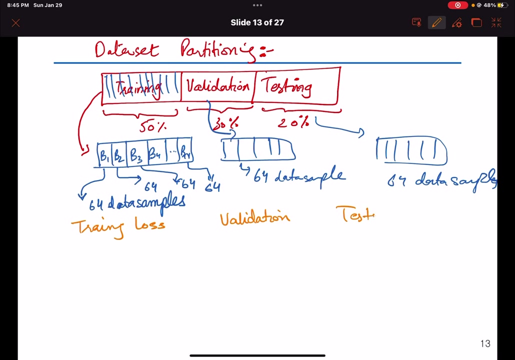 data. And then comes the discussion about your training loss, validation loss and testing loss. So in the training time what you do is each data sample is given one by one to your training model. first you give your first batch, then you give second batch. batch means sample number one to sample number 64.. batch 2 means 65. 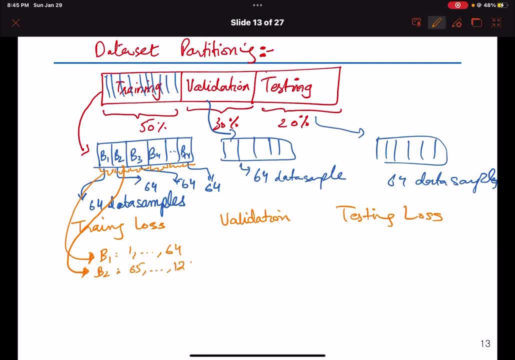 to 129, for example, 128 batch 3, 129 to onwards. similarly, your validation data will also be given input like this. so same is the case with your testing data. so at the training time, what you do is you enter your data batch by batch. so for first batch you have a loss. 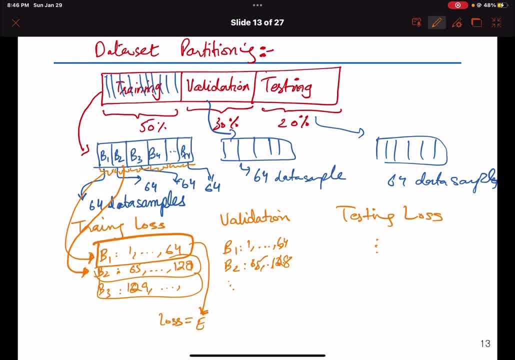 estimated, which we studied, was this: you have to you estimate the loss and then, using this loss, you updated your weight values, for example, using gradient descent learning rate. partial of your loss function with respect to your weight values. so you update your loss at each batch, for each batch. 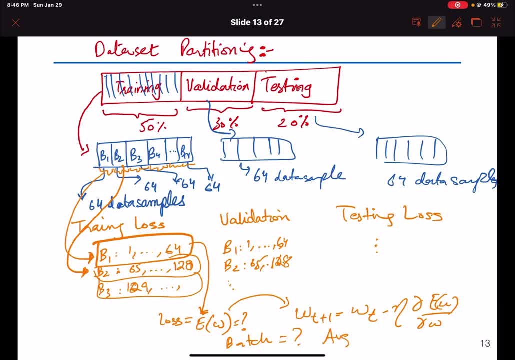 and then what you do is you estimate the average training loss, which is the average of all the loss of loss of batch 1, loss of batch 2 up to loss of batch n, when we have input into our model and update, and each batch will update your weights. 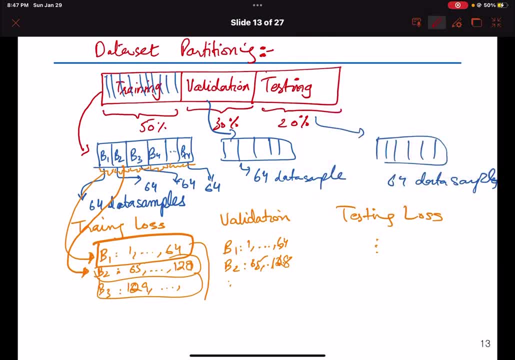 so after each batch, after each batch, your weight values are updated and we call this depending on your loss function and estimated loss. and the loss estimation is here is the training loss, so it is estimated per batch, and then one batch when all of your patches are given as input. 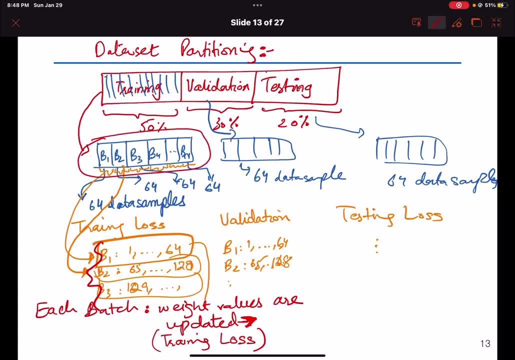 whole of this data is given and your models are updated n times. weight values are updated n times because we have n batches. we call this one epoch, when all your data, training data, is input one time and your weights are updated n times. we call this an epoch- 1 epoch. 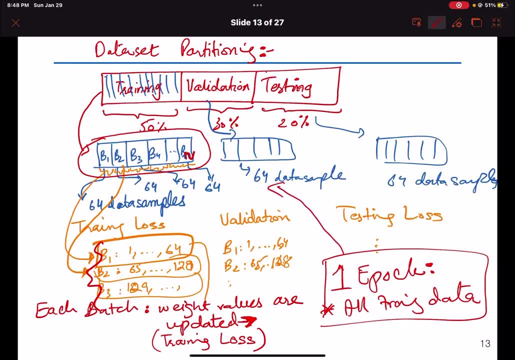 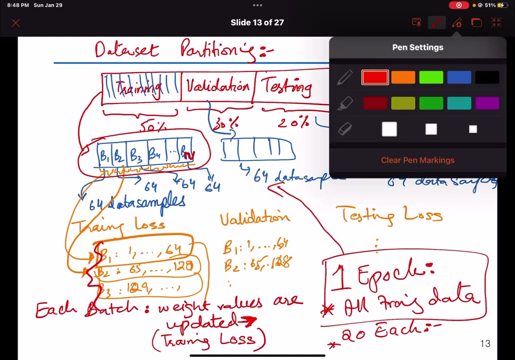 after each epoch we estimate your validation loss. and then, for example, you have 20 epochs, so your model will again be updated 20 times, and every time your weight values will be updated, and after each epoch you will have your validation loss. here i would like to mention something. 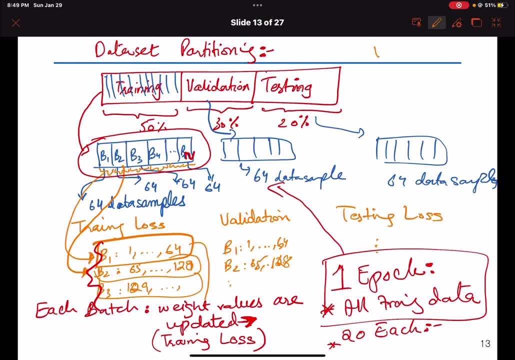 then for your validation loss estimation, your rates are not updated. it is used just to evaluate your model only. the model are updated at training time, only training time. at validation and testing time, the model weights are not updated. and when we have completed the epoch we will have your test data. 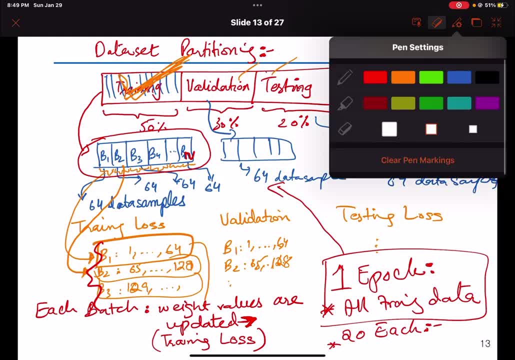 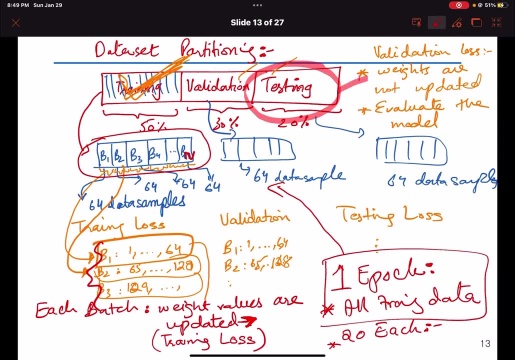 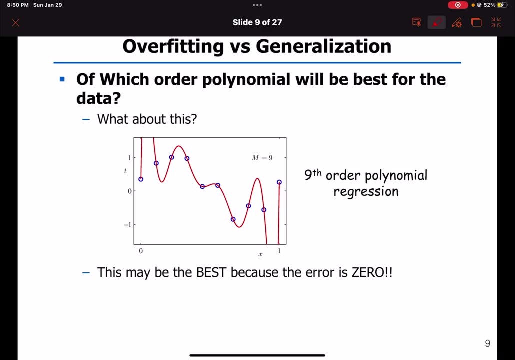 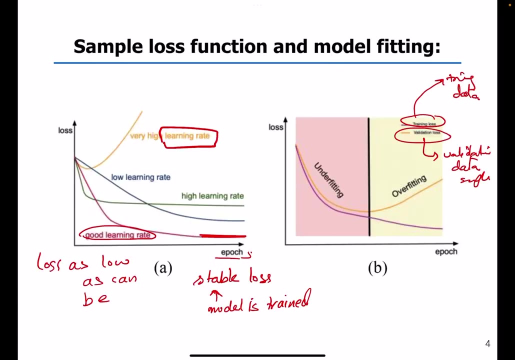 when all of the data set is complete, we will have your test data and we can estimate the testing loss where the weight values are not updated. so the concept we studied here, the training loss and your validation loss. so training loss is estimated per batch and validation loss is.